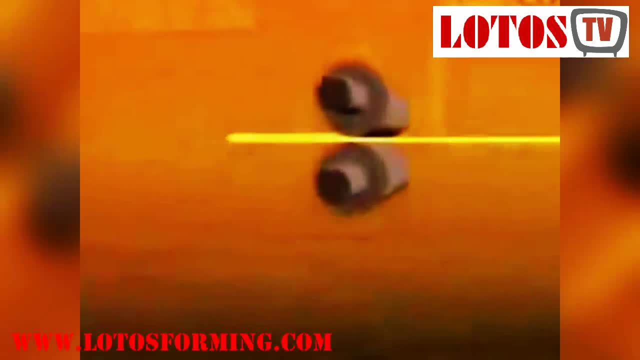 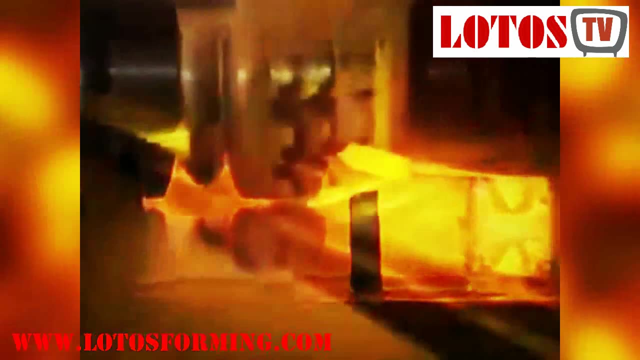 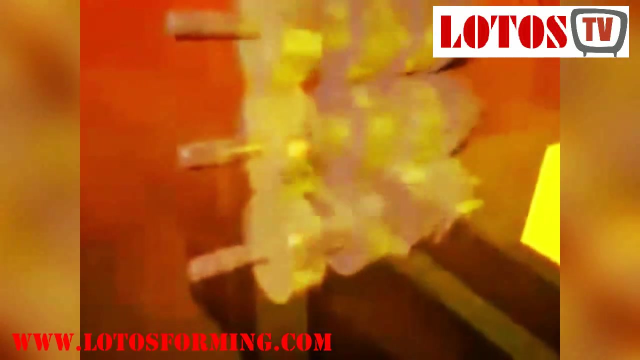 For example, hot rolled steel is used in situations where precise shapes and tolerances are not required. Hot rolled steel typically requires much less processing than cold rolled steel, which makes it a lot cheaper. Because hot rolled steel is allowed to cool at room temperature, it's essentially normalized, meaning it's free from internal stresses that can arise from quenching or work hardening processes. 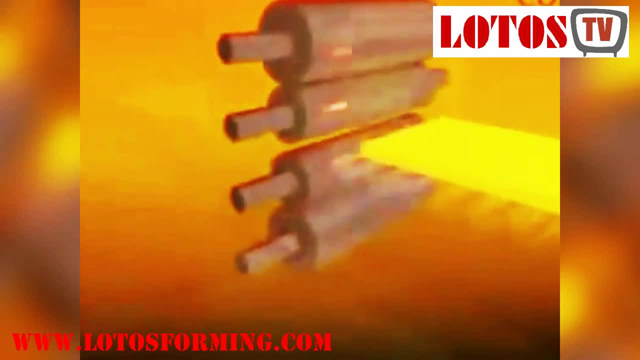 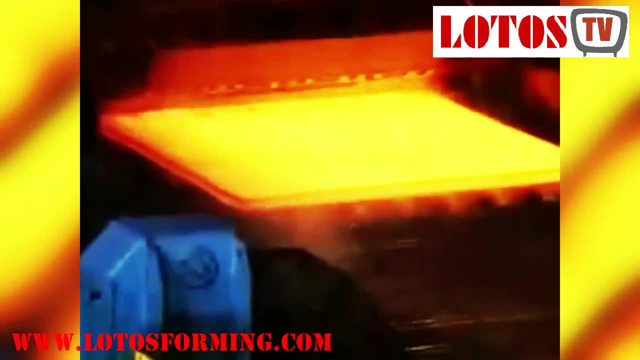 Hot rolled steel is ideal where dimensional tolerances aren't as important as overall material. For example, hot rolled steel is used in cases where material strength and wear surface finish isn't a key concern. Where surface finish is a concern, scaling can be removed by grinding, sandblasting or acid bath pickling. 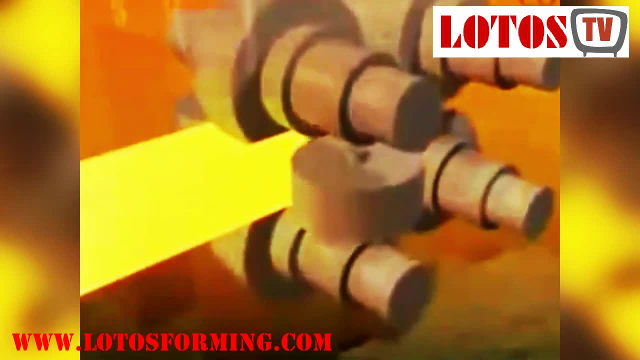 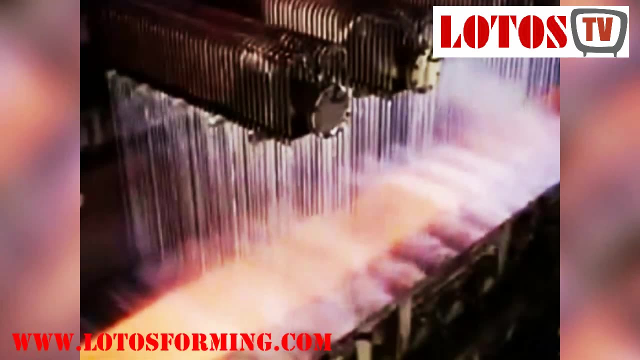 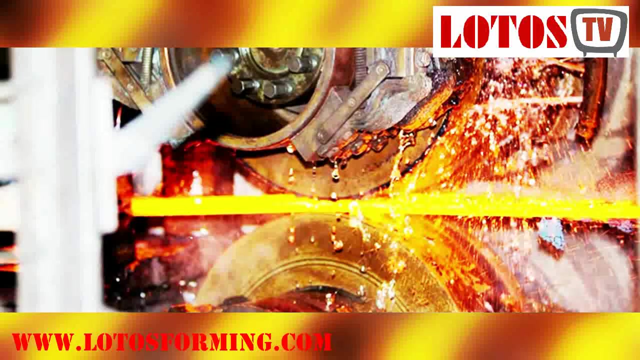 Once scaling has been removed, various brush or mirror finishes can also be applied. Descaled steel also offers a better surface for painting and other surface coatings. When cooling steel after hot rolling, you should expect the steel to shrink slightly. You may find that you have less control over the final size and material. 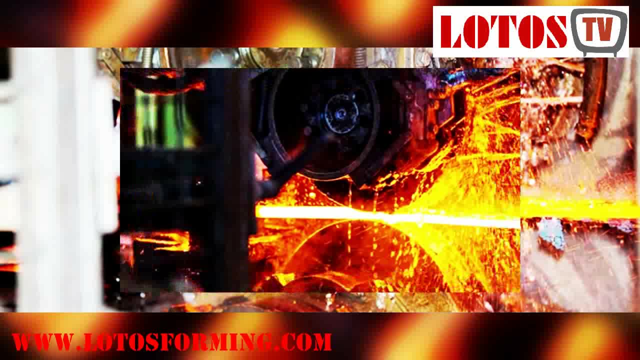 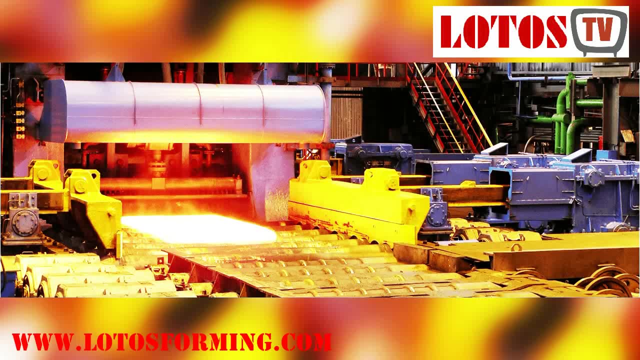 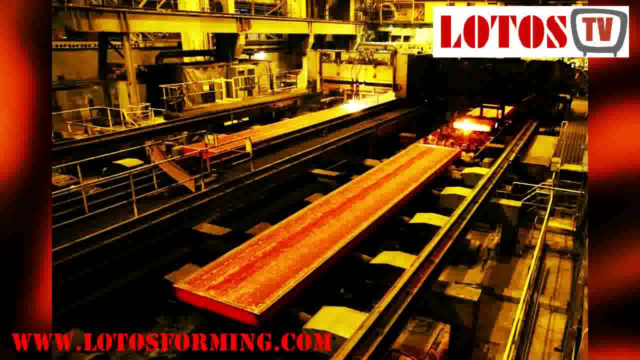 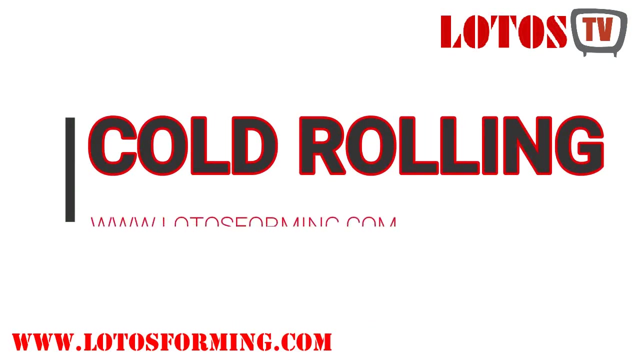 You may find that you have less control over the final size and material When using a hot rolling method. hot rolling, however, allows steel to be formed into much larger sizes than cold rolling When using a hot rolling method. hot rolling, however, allows steel to be formed into much larger sizes than cold rolling. 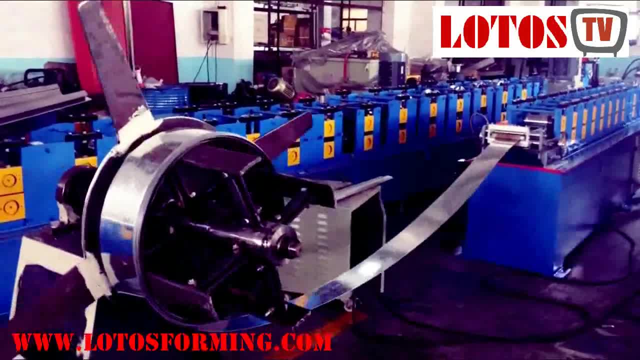 Cold rolled steel is essentially hot rolled steel that has been through further processing. Cold rolled steel is essentially hot rolled steel that has been through further processing. Once hot rolled steel is cooled, it is then re-rolled at room temperature to achieve more exact dimensions and better surface qualities. 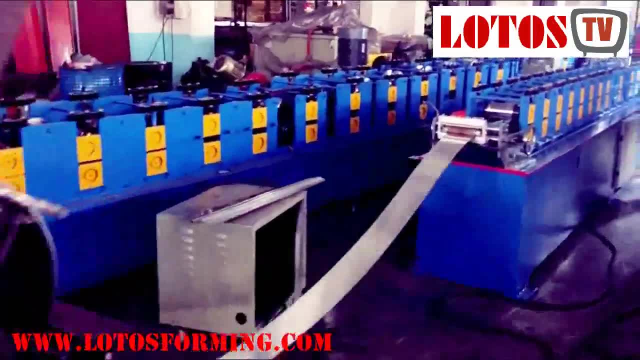 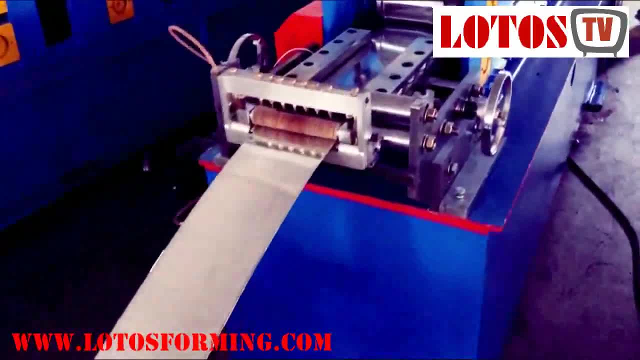 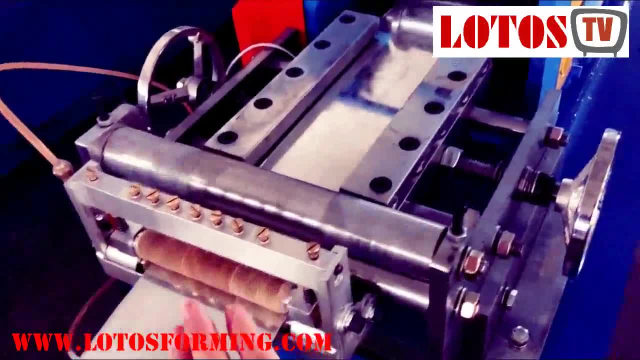 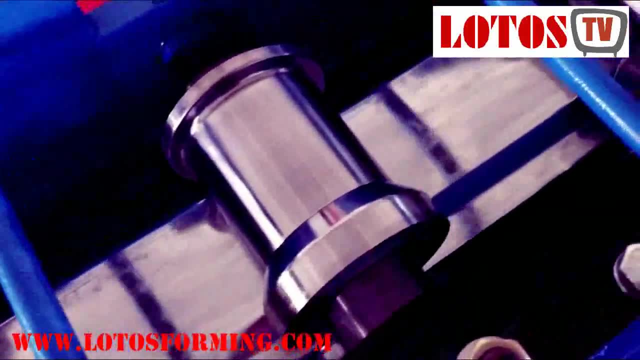 Cold rolled steel is often used to describe a range of finishing processes, though technically cold rolled applies only to sheets that undergo compression between rollers. describe a range of finishing processes, though technically cold rolled applies only to sheets that undergo compression between rollers. Steel forms that are pulled, such as bars or tubes, are drawn, not rolled.